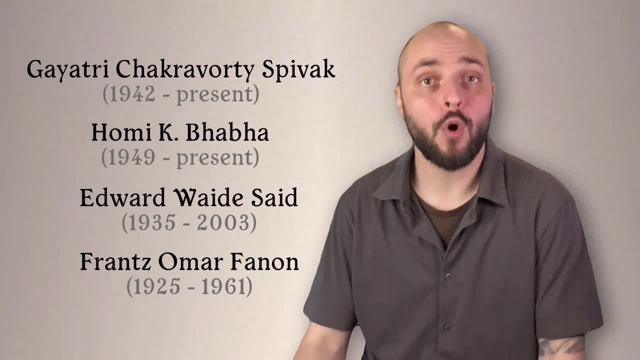 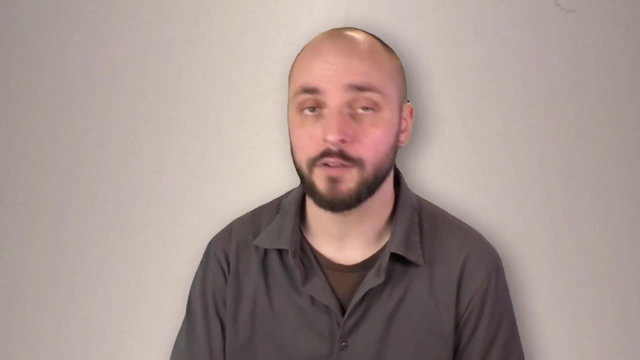 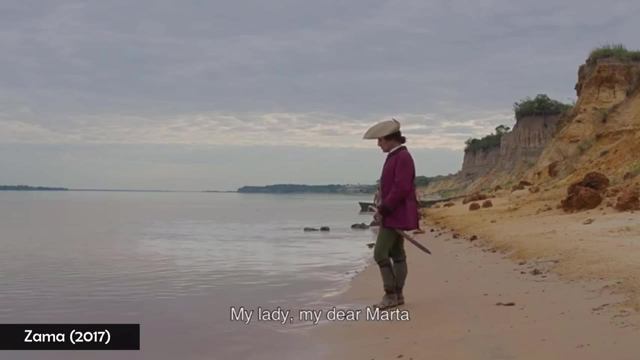 Fanon's writings form what many consider to be the core of postcolonial theory and, taken together, this huge body of writing, which includes contributions from political philosophy, linguistics, sociology, feminism, critical theory and cultural studies, works to promote new forms. 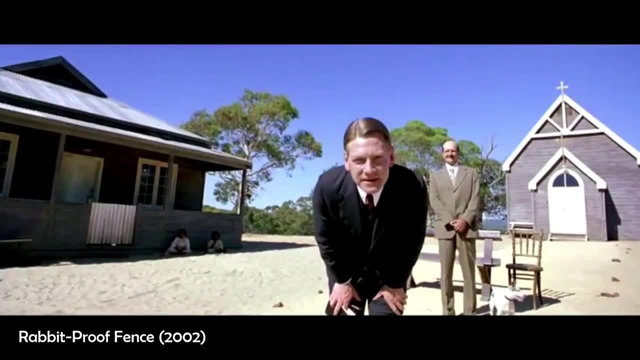 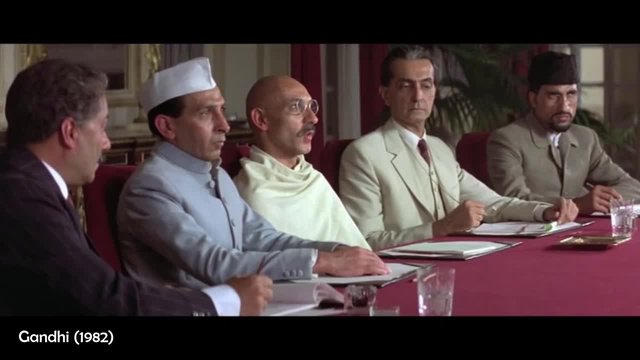 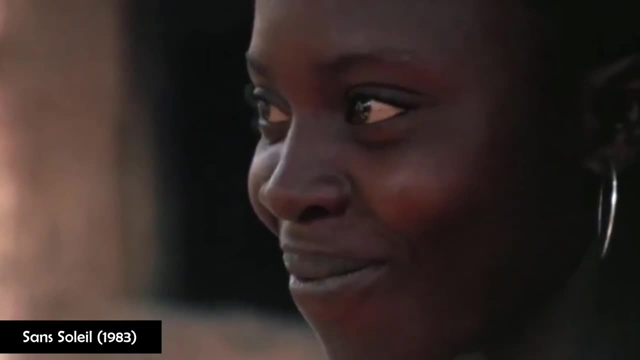 of inquiry into the colonial past, as well as advocating anti-colonial resistance today through cultural criticism, the promotion of postcolonial voices and direct political action. In that sense, postcolonialism doesn't have a single founding figure, but rather grew out of. 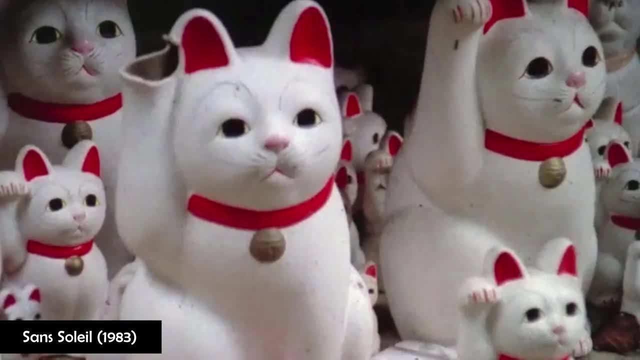 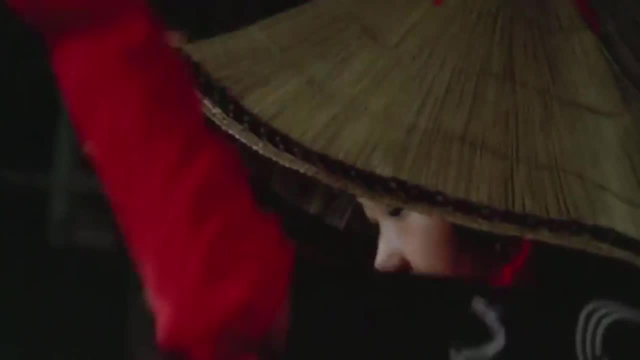 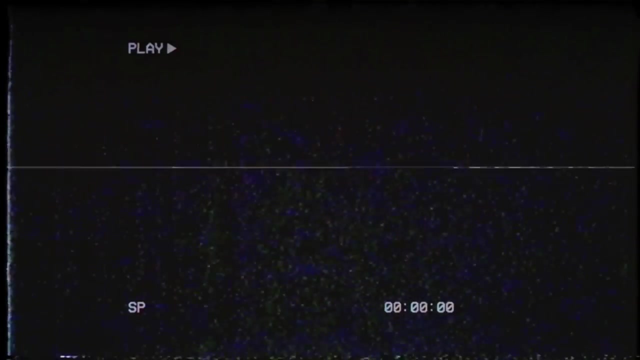 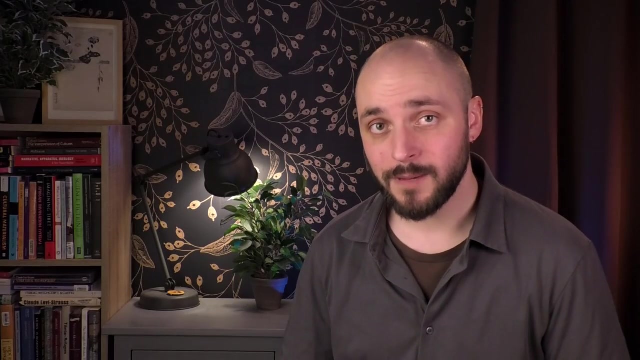 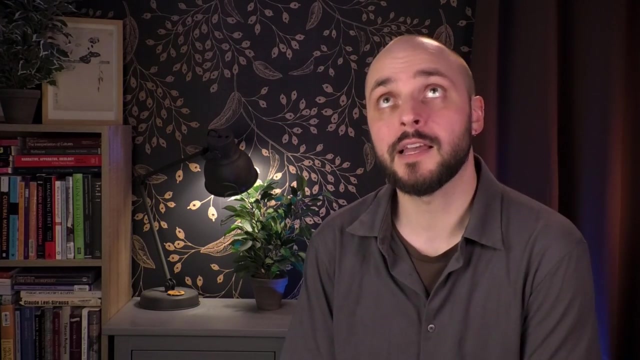 anti-colonialism. So what are some common criticisms of postcolonial theory? Well, one of the major ones- and this may sound strange- is that it's very difficult to read. A number of postcolonial thinkers, like Gyatri Spivak, were heavily influenced by postmodern literary. 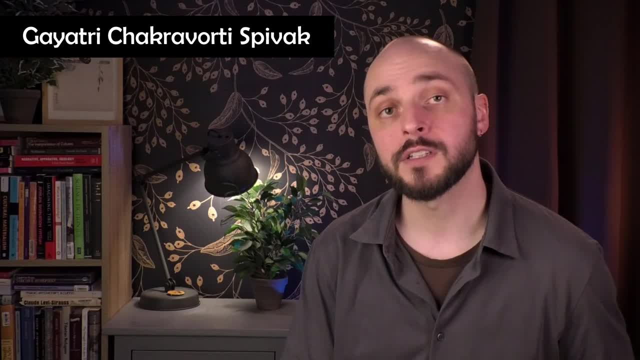 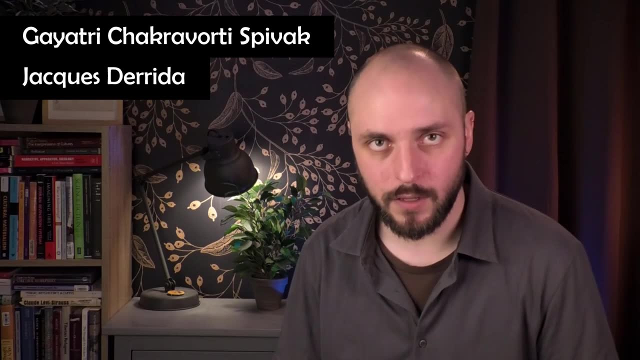 criticism, particularly by Deconstructuralism and the works of Jacques Derrida. This made their writing extremely dense and full of technical jargon that's impossible to understand without also reading postmodern literary theory. That's something that a lot of people complain about. 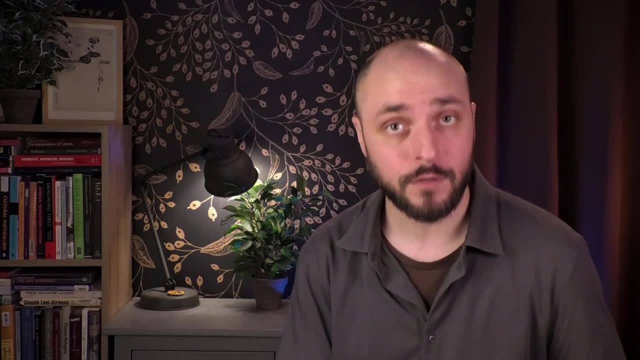 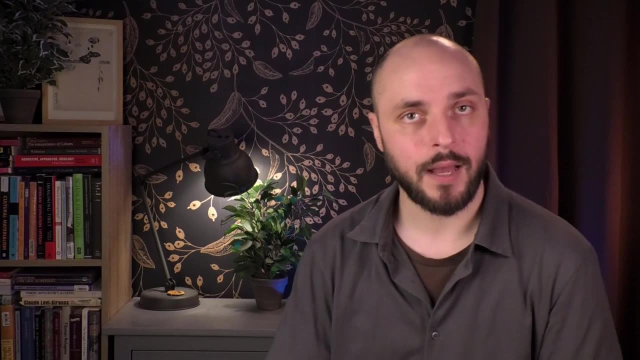 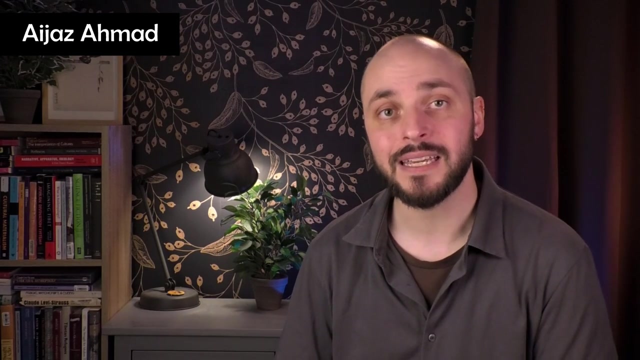 and it really does make some of the field's core texts difficult for students. That's a definite downside. Postcolonial academics have also been criticized from the left and by non-Western scholars, like the Indian author Ajaz-e-Hamad, for publishing extensively, sometimes entirely, in English. 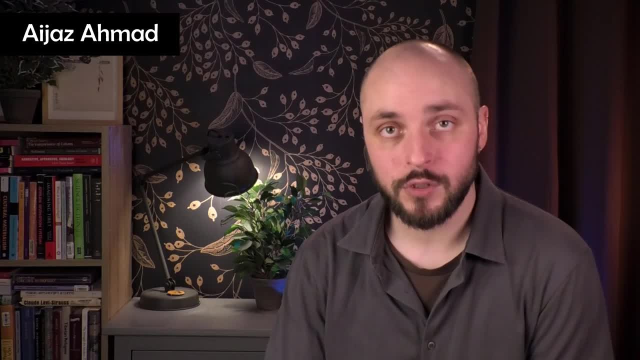 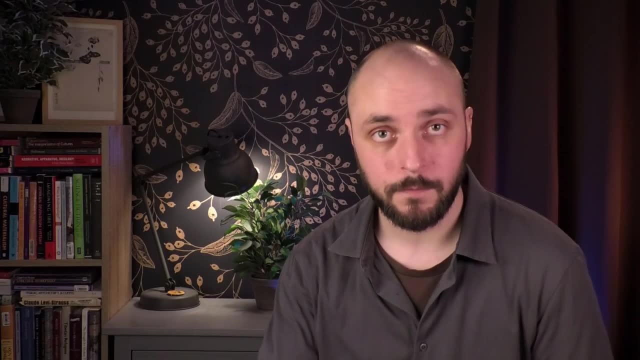 and neglecting to translate their work into the indigenous languages that are often spoken in postcolonial states, For example into Arabic, Hindi, Urdu and Yoruba, And that has sometimes called into question the political commitment of some postcolonial authors. But the most strident, the most pronounced criticism of postcolonialism has definitely come from the European and North American conservative movement, not just the right wing but also traditional conservatives on the center-right, And their criticism is much the same as it is with. 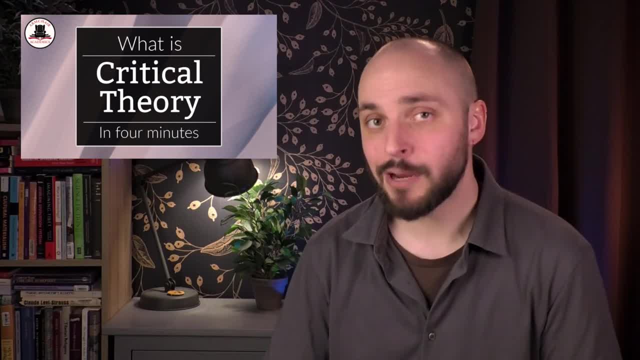 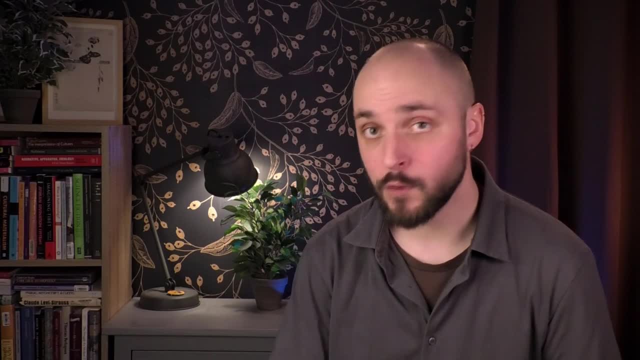 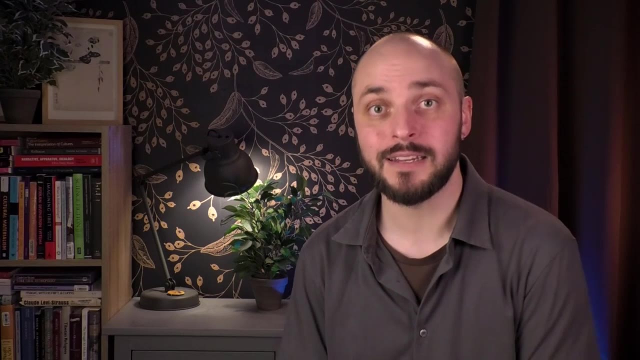 critical theory that postcolonial scholarship introduces a radical and anti-Western agenda into universities that aims to undermine the political and economic hegemony of the West. Now, postcolonialism ranges from the ridiculous that simply being exposed to non-Western ideas will.